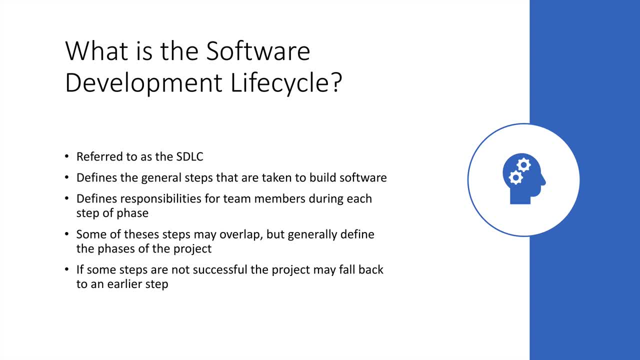 by software development teams. The SDLC defines the responsibilities for team members during each step of the phase. Now. some of these steps may overlap, but they generally define the phases of the projects. Also, if some of the steps are not successful, the project may fall back to an earlier. 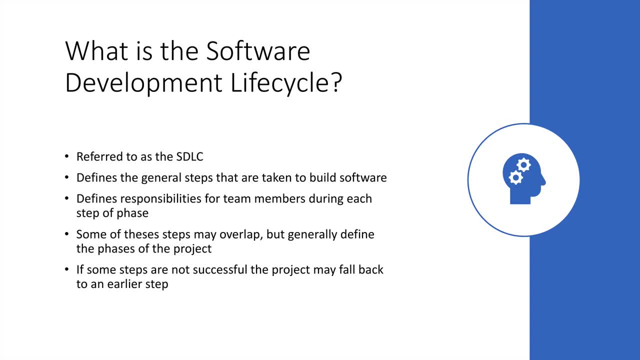 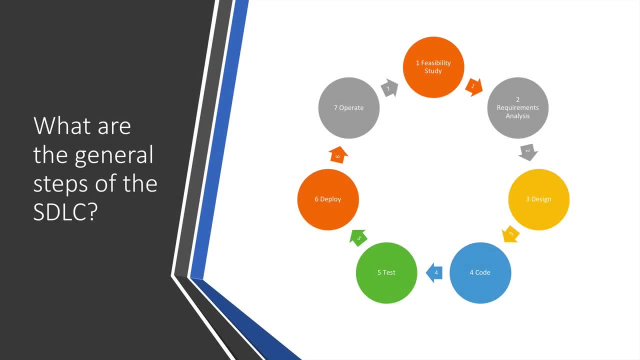 step. So let's go ahead and look at the details of the steps of the SDLC. So what are the general steps of the SDLC? The first step is a feasibility study. Step two is the requirements analysis. Following that is the design phase. 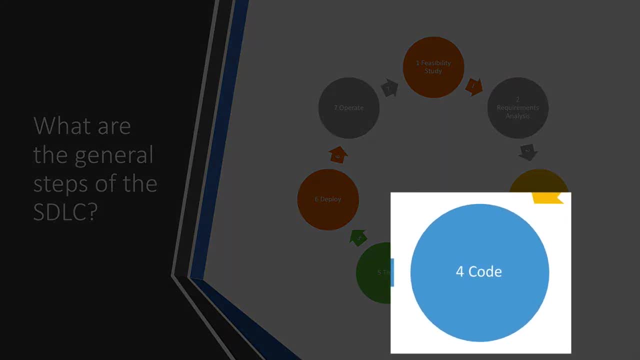 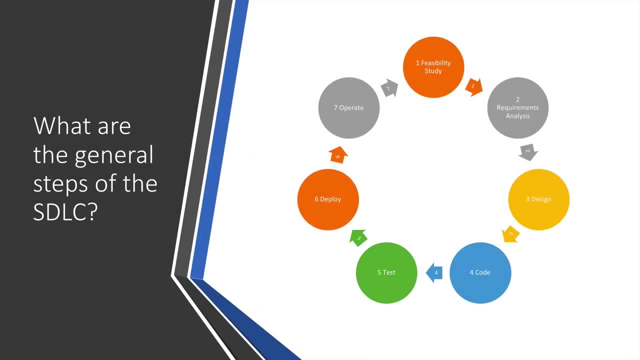 Next is the coding phase, which we're all mostly familiar with, when programmers are actually producing code. Followed by that is the testing stage. Once the testing has been successfully completed, we move on to a deployment stage, where code is actually put into production And the 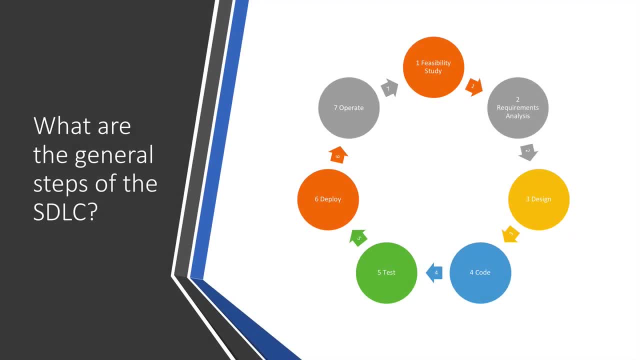 final stage is the operational stage, where maintenance teams and support desk people are supporting the operating software. So let's look at each one of these steps in a little bit more detail. The first step in the process is the feasibility study. Step two is the development. 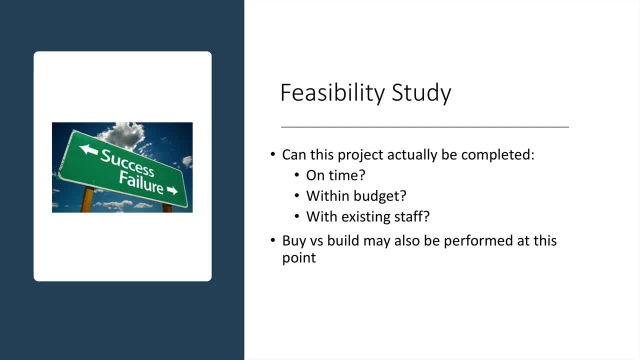 phase. The project team will want to answer some key questions at this point. For example, can the project be completed on time and can it can be completed within the existing budget that's been set aside for this particular project? Also, with the existing staff do you have the expertise in? 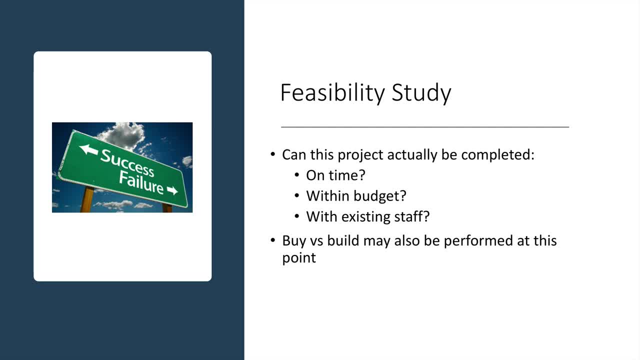 house to do this kind of project, or are you going to have to hire out contractors? Another key decision that's made at this point is a buy versus build decision If you have the expertise in house to do this and that doesn't require modernized software, which isn't necessarily the best. 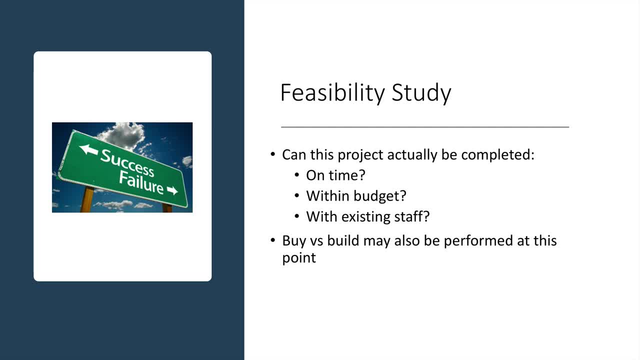 ognition at this point. Is there a relatively customs type of software? do you go ahead and build that with internal staff, or is there an existing software package that you can buy off the shelf that meets your needs? So that's really it for the feasibility study. let's go ahead and move on to 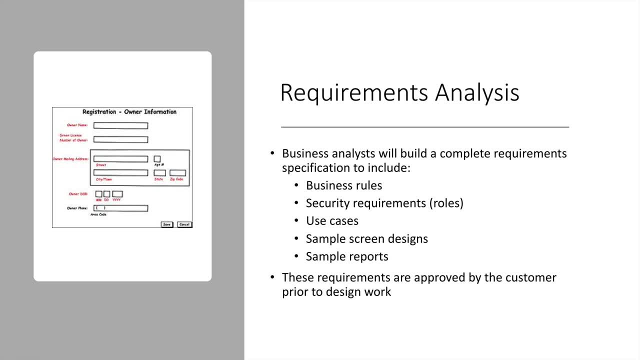 the next step. The next step in the process is the requirements analysis. In this phase, business analyst will build a complete requirement specification that includes business rules for the access to the system. You'll look at use cases, common scenarios of how people are going to use the system. They'll generate sample design screens and walk through. 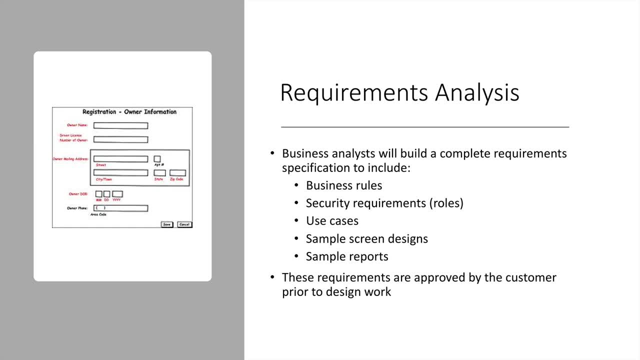 that with the potential users to make sure that the system will meet their needs. And also sample reports are important at this point because reports drive the kind of data that needs to be set into the system. They're very important to design at this point so that you make sure that you don't. 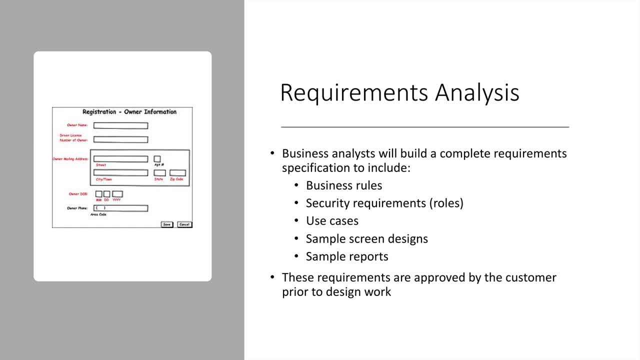 overlook any details. Once you get to the coding or operational phase and you find out that you've left out some data details, it becomes very expensive to rework and redesign the system. These requirements need to be approved by the customer with a formal approval before work begins on the system. So 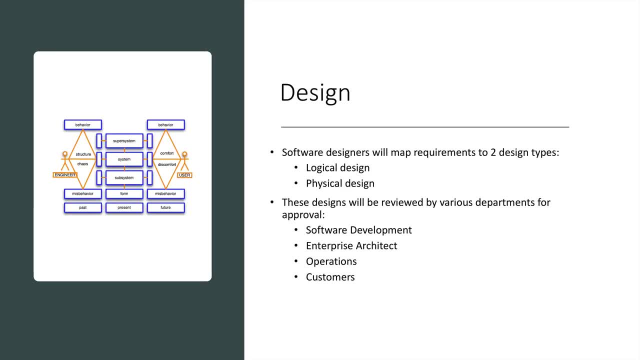 that's it for the requirements analysis. Let's move on to the next step. The next step is the design phase. In this phase, software designers will map the detailed requirements into two major details. The first is the design phase, The second is the 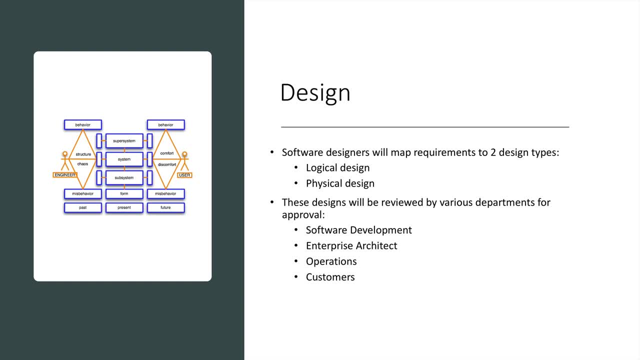 design types. The first is a logical design: That's how the general components will fit together and what is the overall hierarchy of that design. The next type of design is a physical design, and this will be detailed things such as database schemas that lay out the individual fields and table in the 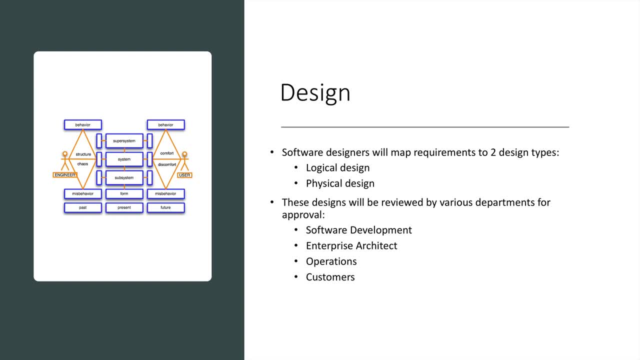 database and their relationship. These designs will be reviewed by various departments and it depends on the size of the company, but it will be reviewed certainly by software designers, Software development management, an enterprise architect- if there is an enterprise architecture and most large companies have this type of capability. 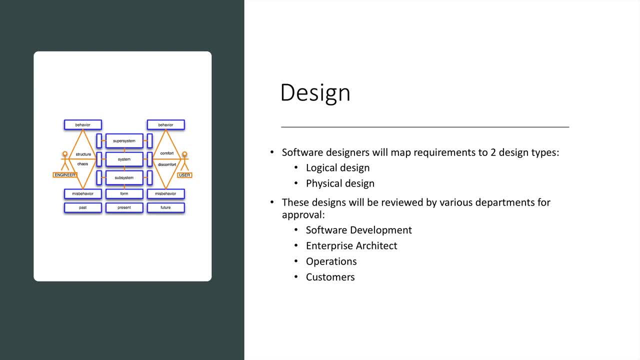 Also be looked at by operations personnel to make sure that they can operate the software and support it effectively. and also, these designs will be reviewed by the customer to make sure that everything has been accounted for. So that's it for the design phase. Let's move on to the next step. The next step. 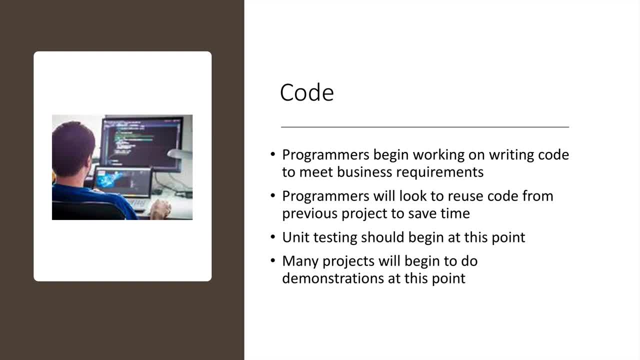 is the coding phase, and this is the phase that we usually associate with software development. So programmers will begin to work on writing code to meet specific business requirements. at this time. The code is highly targeted to meet specific requirements that are generated from the earlier steps In. 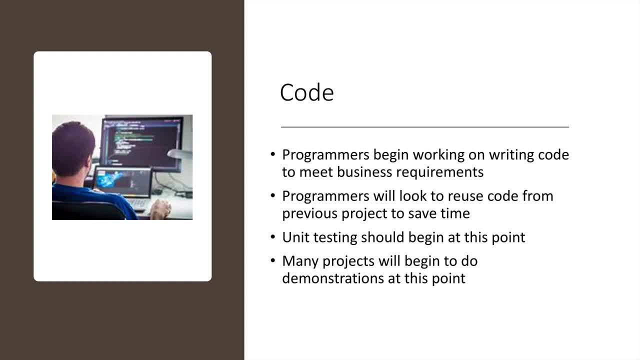 addition, programmers will look to reuse code from previous projects to save time. Also, unit testing will begin at this point. So, as programmers write individual pieces of code, they will build tests that they can run in an automated way To make sure that the system is functioning as expected, and they'll layer. 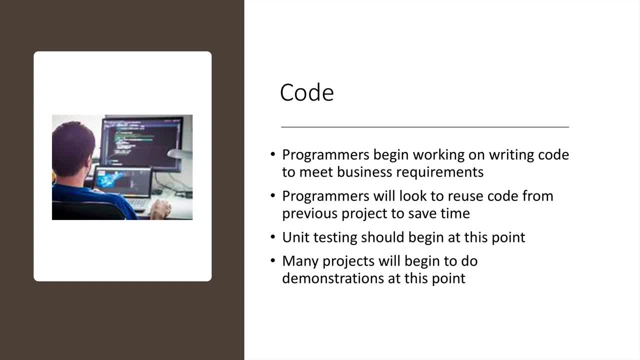 these tests from the bottom up, as they're building code so that they can retest the system at any point. In addition, many projects will also begin to do demonstrations at this point to the customers. They want to make sure that the software is meeting the needs of the customers and that nothing is overlooked. 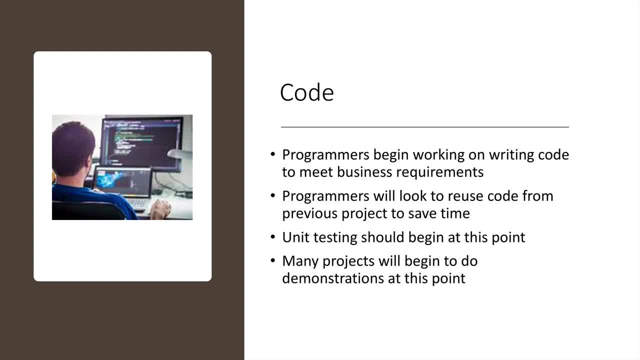 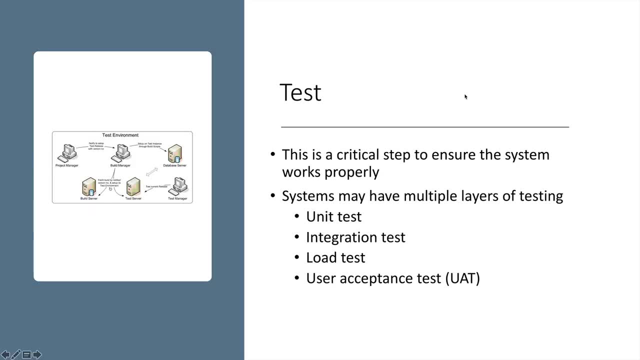 So nobody likes surprises, particularly at the end of the project. So that's really it for the coding phase. Let's go ahead and move on to the next step. The next step is the testing phase. So this is a critical step to ensure that. 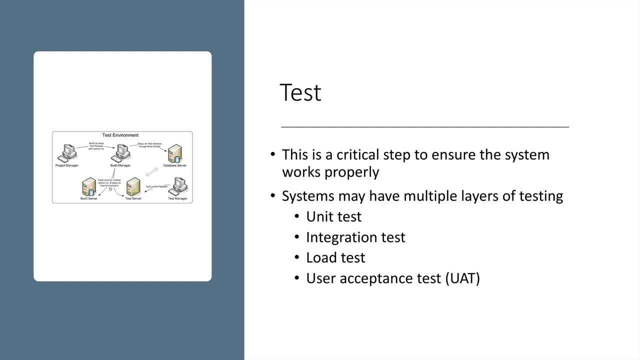 the system works properly. We've seen lots of examples over recent years of systems that were deployed and weren't tested properly, and it's very difficult to recover from that, trying to operate the system that has lots of bugs, Or perhaps it wasn't load tested properly and you get way more usage than you. 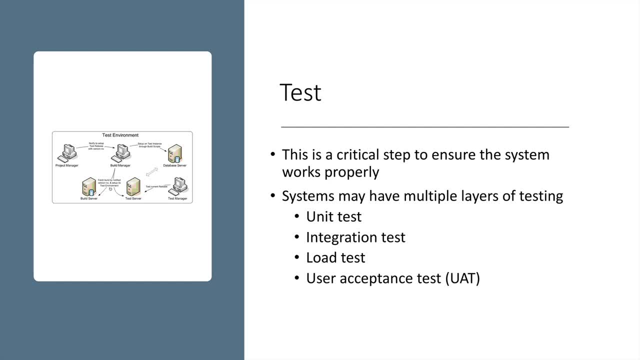 thought you. The system begins to fail in multiple ways, So there are multiple layers of testing. The lowest level is the unit test, and programmers will develop these while they're coding. Integration test happens to test interfaces to other systems, so as bigger components. 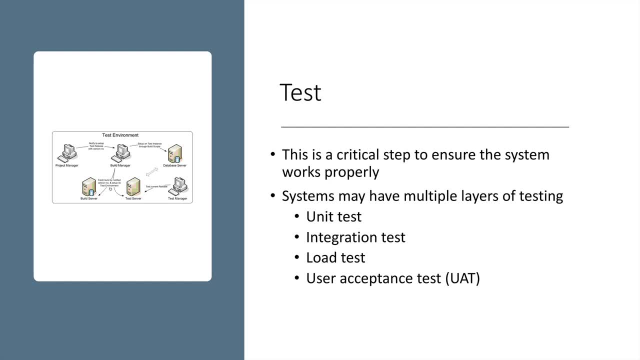 of the system are completed, integration testing will happen to make sure that those interfaces work properly. The next type of testing is load testing to make sure that your system can support the anticipated number of users that are going on in the system. There's been a number of high profile failures over the last few years where systems were 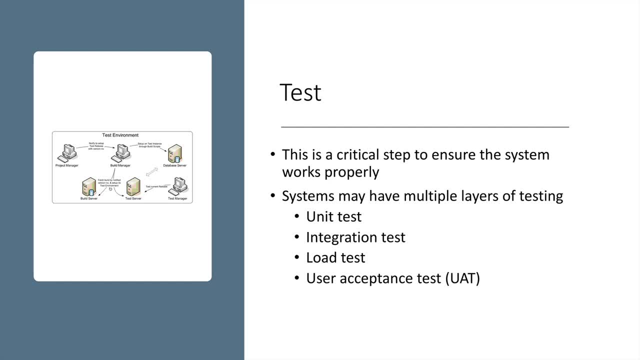 rolled out with lengthy delays, performance problems and a real lack of user confidence in the system. when you see these types of problems, Also, user acceptance testing happens, where the actual users of the system will sit down before the system is released to make sure that it meets their needs. 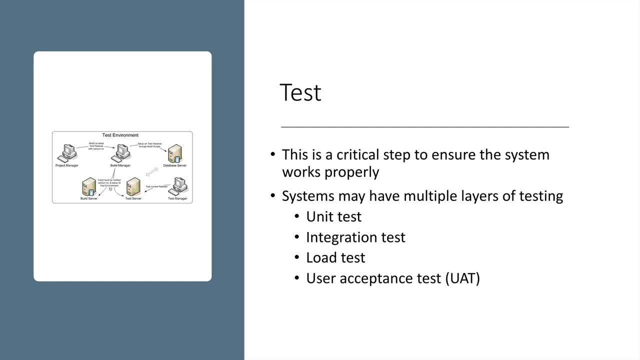 That's really it for the testing phase. Overlooking this phase can be very difficult to produce a quality product, so enough time and money needs to be invested in testing to make sure that your system launch is going to be successful. Again, that's it for the testing phase. let's move on to the next step. 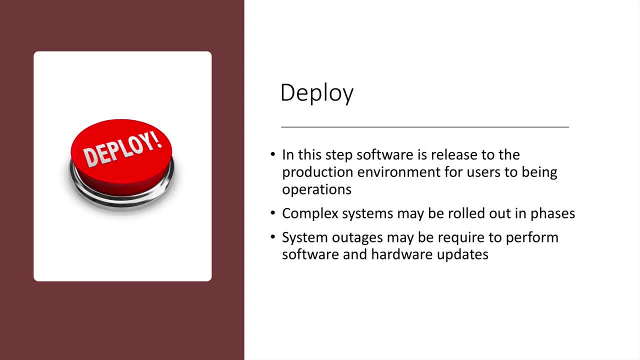 The next step is to deploy the software into production. So in this step software is released to the production environment for the users to begin operations. Complex systems may be rolled out in phases. if it's a really large system, maybe pieces of the system are rolled out one piece at a time in a phased approach to limit the risk. 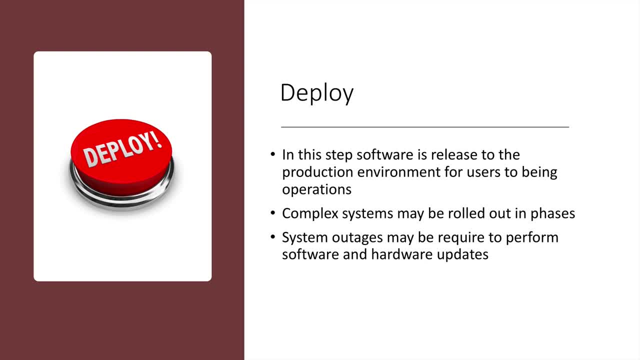 of having too large of a system to roll out and having too many problems to address. in that phase, System outages may be required to perform software and hardware updates. so a lot of times these types of deployments are done off hours. maybe it's done on a holiday weekend. 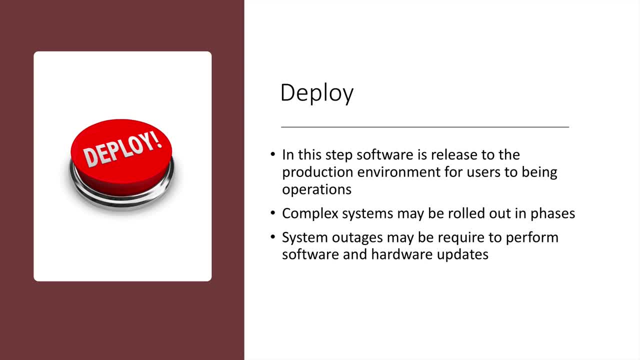 or late at night or very early in the morning. So you want to deploy the software when there is very limited usage on the system. So that's it for the deployment stage. let's go ahead and move on to the last step of the process. 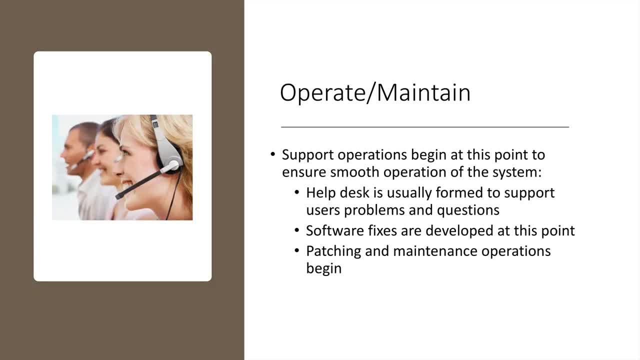 So the last step of the process is the operational and maintenance phase. Support operations will begin at this point. to ensure the smooth operation of the system, A help desk is usually formed to support users and problems and questions as they happen, as well as operational support from the software and development teams. 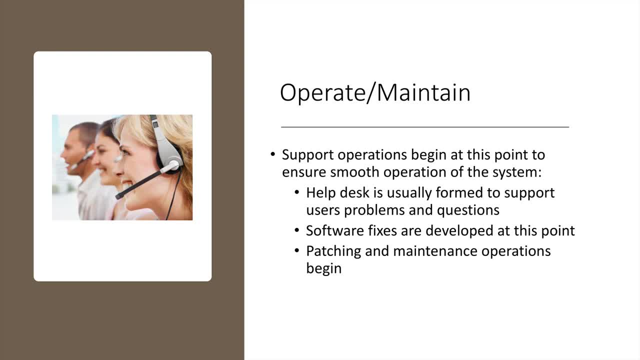 Software fixes are developed at this point and routine patching and maintenance operations begin. So things like patching, operating system updates, routine software updates and routine software updates- All of these things occur during the operational and maintenance phase. So that's the last step of the process. so let's go ahead and look at a wrap up of the 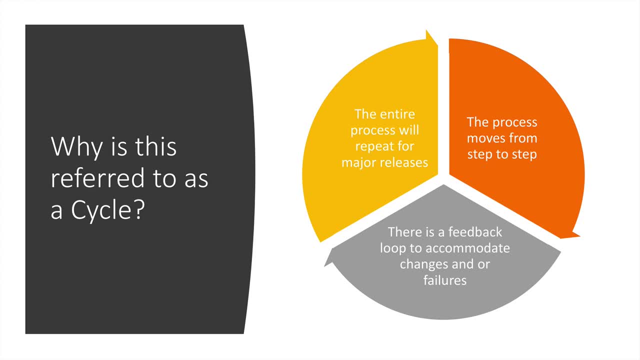 SDLC. So why is the SDLC referred to as a cycle? The process moves from one step to the other and there's also a feedback loop to accommodate changes and or failures. So if you fail in one particular step, so maybe you run into problems in coding you. 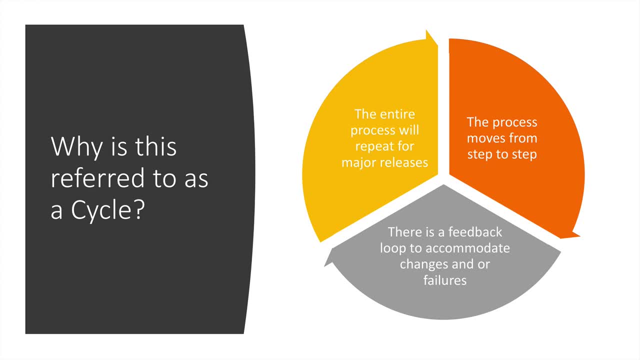 may have to move back to the requirements analysis. You may have to go back to the requirements analysis phase to fix that Also. the entire process will repeat itself for major releases. So once you're in operations, many of your users or your business will change and there 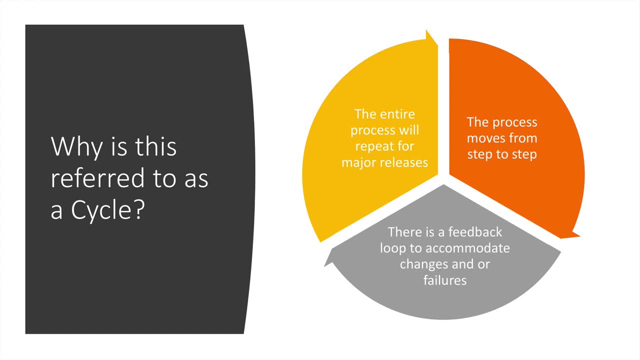 are anticipated new features that need to be developed for the system, So the entire process will start all the way over again for the next release. So that's really it for the software development cycle. Let's go ahead and look at the summary of what we've talked about in this lesson. 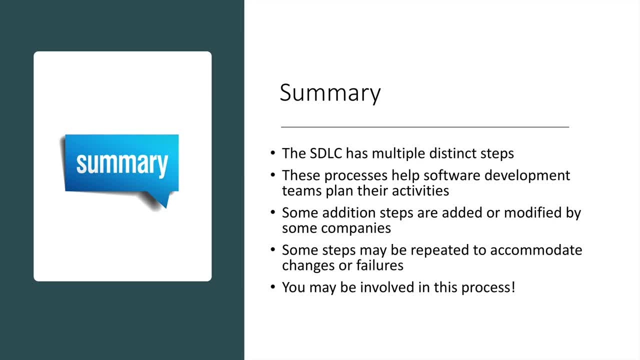 In summary, the SDLC has multiple disciplines, Multiple distinct steps or phases. These processes help software development teams plan their activities. In addition, some companies may add additional steps that meet their specific needs. They may have particular processes that they have found to help them be more successful.